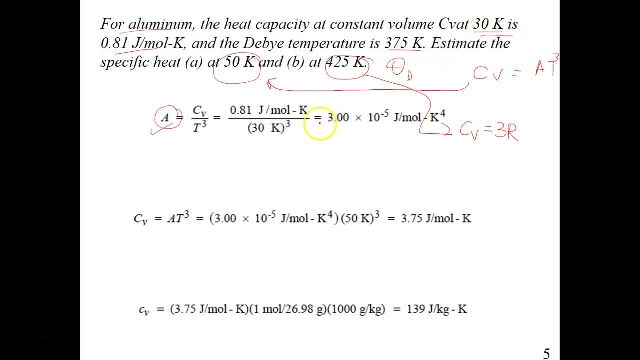 of 3, you will use this 30 Kelvin, So you will get your A. And then, when you got your A, you just substitute in this equation and you know, this is your A that you calculated from here, and this is your 50K, which is: 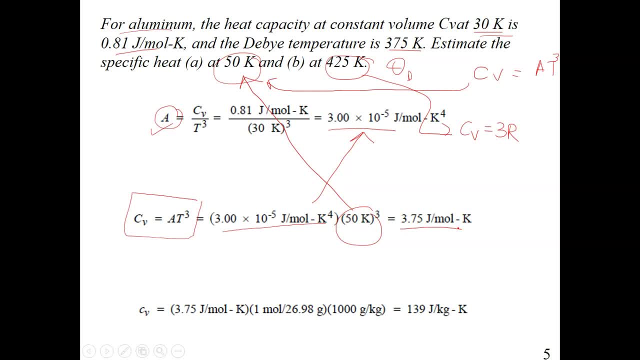 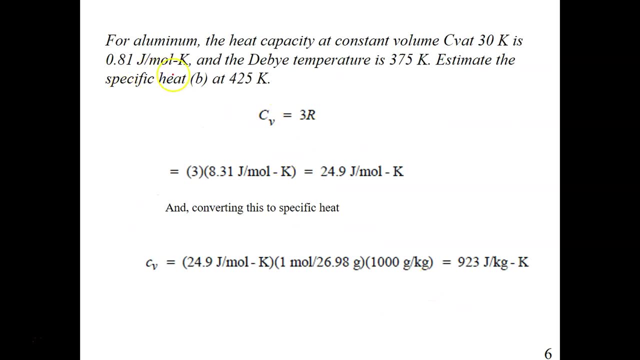 from here and you will get 3.75 joules per mole Kelvin for the answer in A All right. So this is the solution for the second part. So you know that this 4 to 5 Kelvin is definitely more than the Debye temperature, So you need 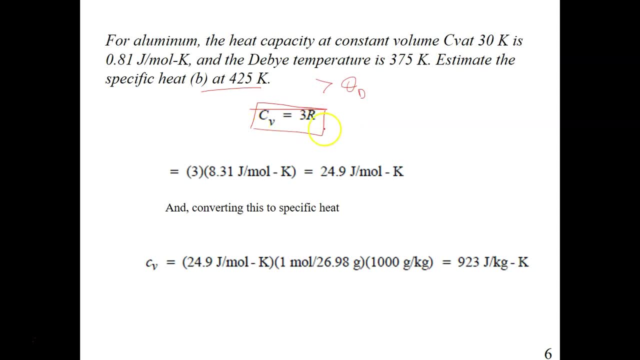 to use this formula, CV equals to 3R, So you may calculate your 3, and this is just simply your gas constant. So this will be your answer, because you know that, more than the Debye temperature, the CV is independent of your temperature. And converting this to 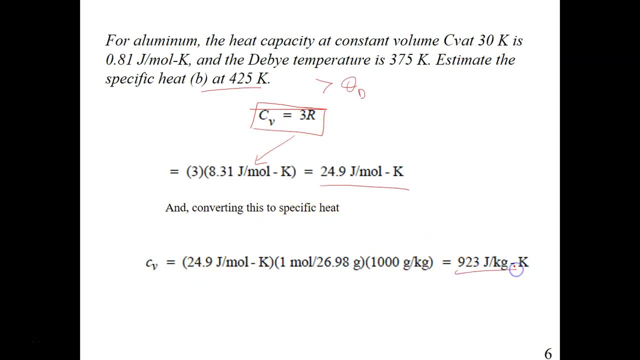 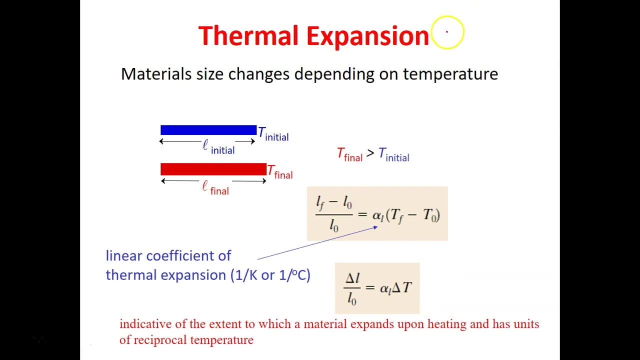 specific heat, you get this All right. Next, we call this thermal expansion. So what is it actually? So usually solid materials. they will expand upon heating and they will contract upon cooling. So that is common sense. I'm sure that you guys can relate to that And the change in the length. 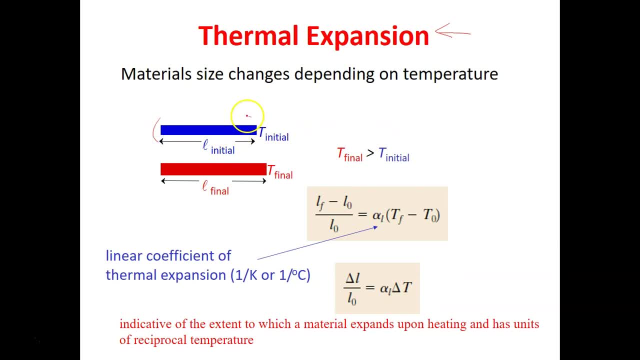 the change in the length. So let's say: this is the heat, So this is the heat, So this is the heat, So this is the original length of your material And after heat is applied, there will be an increase. 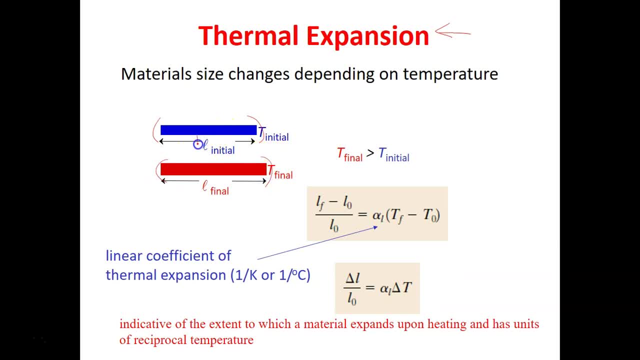 in the temperature, So your material will expand and elongate up to this length. And the change in the length with temperature for a solid material can be expressed using this formula, And this one here The alpha L is- we call it linear coefficient of thermal expansion, and the unit is reciprocal. 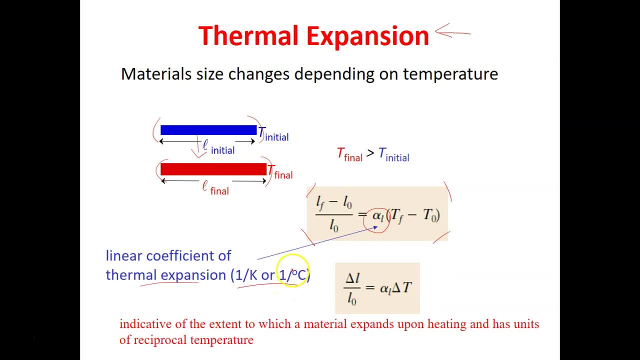 of temperature. All right, The units of thermal expansion coefficient is the reciprocal of temperature, And what is it actually? It is a property. This is a property that indicates the extent to which a material expands upon heating. So it's a property. We will call this the